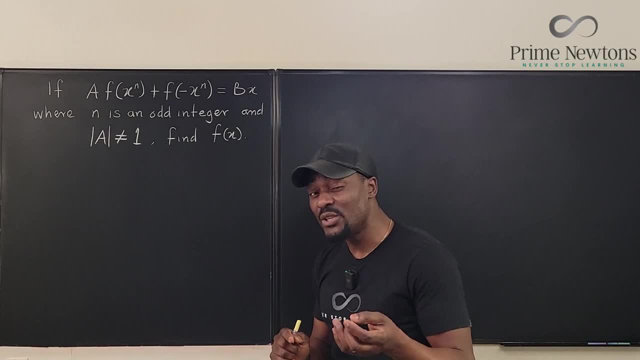 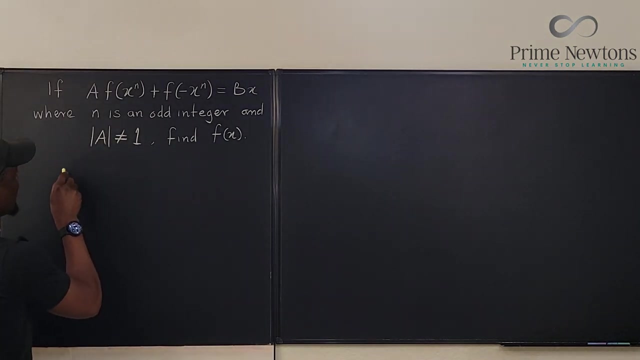 Now, because of the nature of this, I think the fastest or the best thing you want to try first is to play with the signs because of the odd power. So what I'm going to say is I'm going to write: let's do a times f of x to the n plus f of. 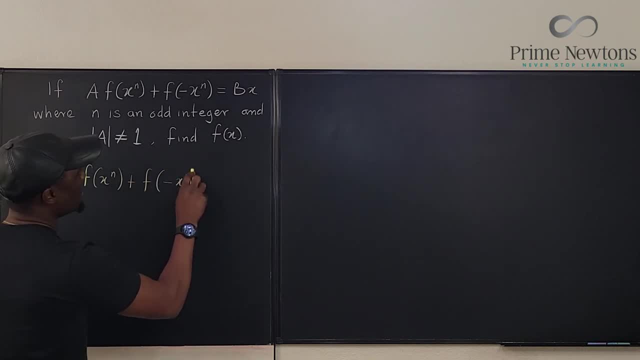 negative 1. Negative x to the n will be equal to b times x. So what I'm going to do next is: I just copied the question. but what I'm going to do next is, instead of plugging in x, I'm going to plug in. 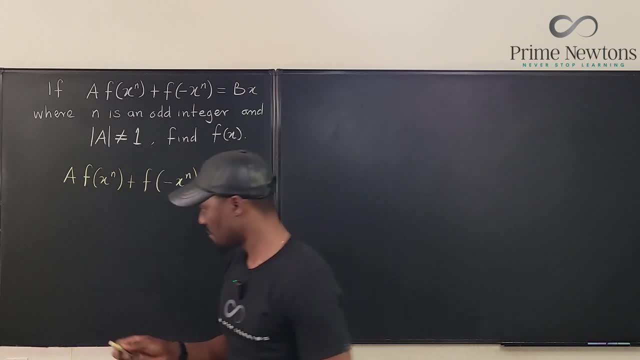 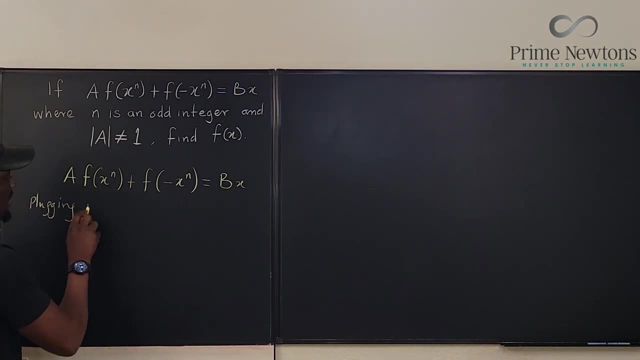 negative x and see what happens. So if I plug in- plug in negative x- I'm going to have a times. a f of this is going to be negative x, raised to power n It's going to be like this: Negative x. 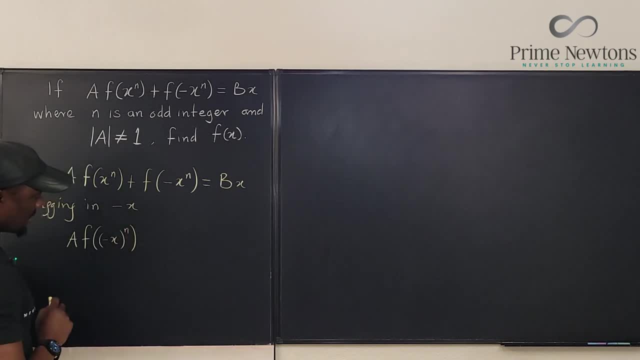 raised to power n plus f of this is going to be negative. and then this would be negative: yeah, x raised to power n. Ah, like this, Let's replace like this: Nice x will be equal to b times negative x. It's going to be negative bx. 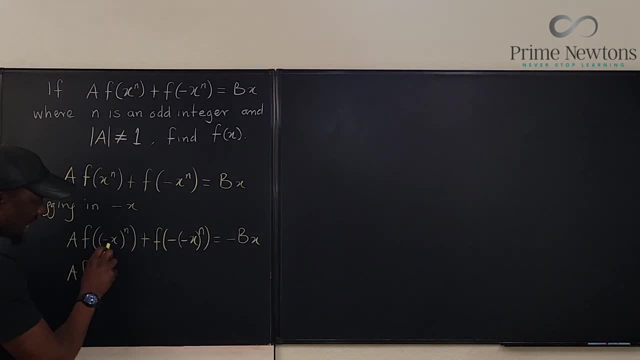 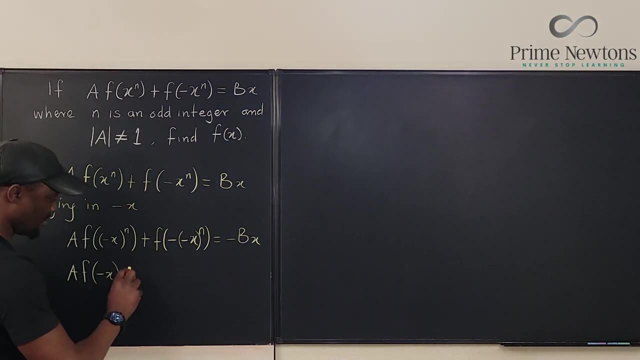 a f of negative x raised to power n- because n is an odd integer- is just going to be negative x. Nothing has changed. Plus, negative x raised to power n will be negative x. but if you multiply again by negative it becomes f of positive x to the n. 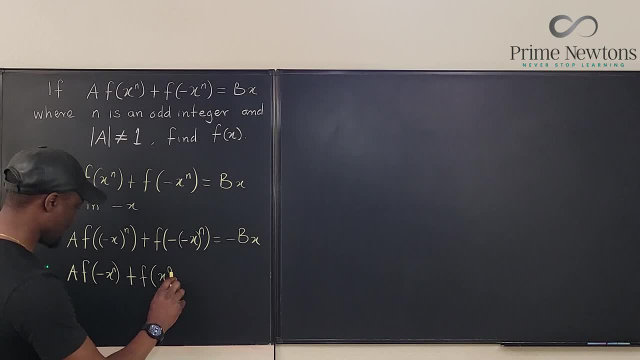 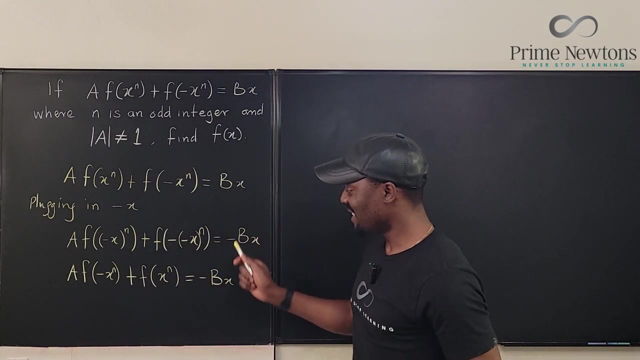 Oh, what is the n here? Come on, Yes, like that To the n. Like that, Okay, And what is left Equals negative bx. Okay, I can see positive bx up here and I can see negative bx up here. 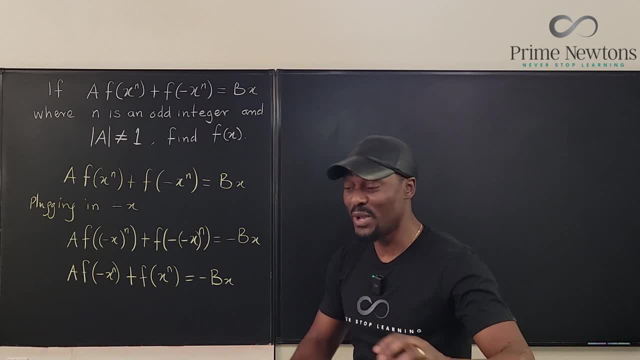 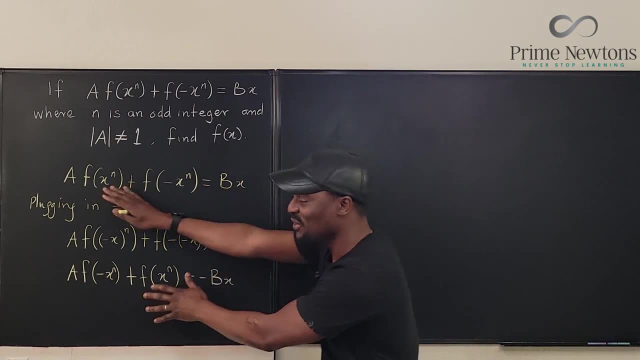 And something about functional equations is: once you see zero, you get very excited. So I'm excited that these two can cancel out. So what I'm going to think of right now is: I don't care what's going on here, but I just want to add this to this so I can get zero on. 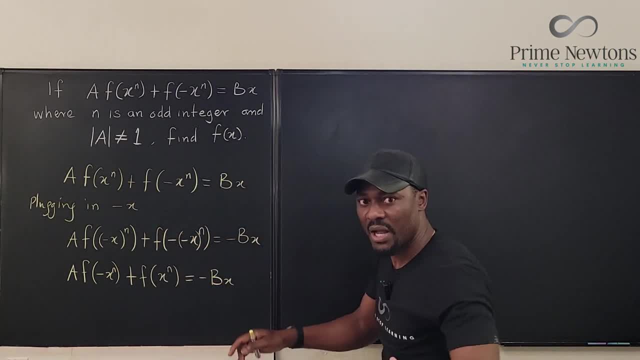 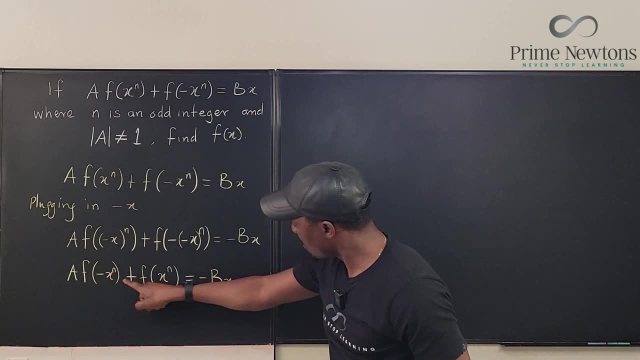 the right-hand side. That means I'm adding all of these together. But if you pay close attention, you notice that f of x to the n is here and it's also here. So it means I'll be adding this to this and I'll be adding this to this. So this is what it's going to look like. 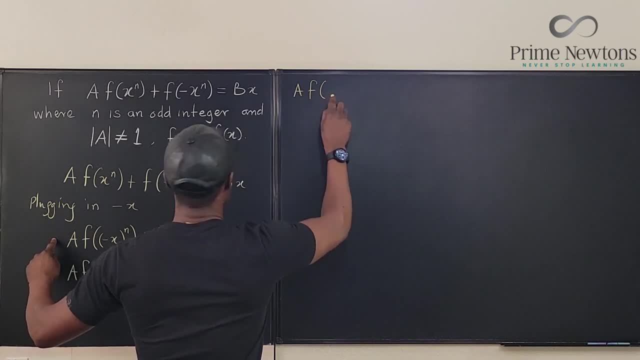 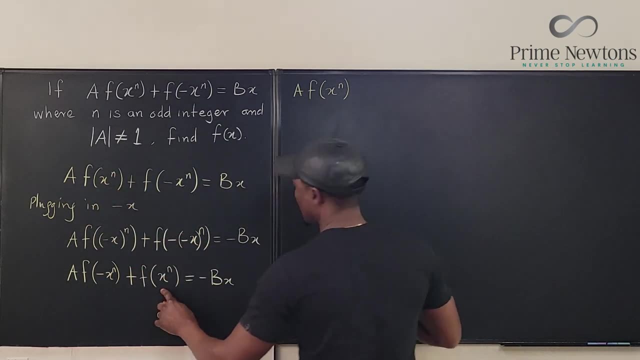 I'm going to have a f- f of x to the n and I'm going to add this to this, and I'm going to add this to this f of x to the n and I'm going to be adding this to this. so I'll add it to this one. 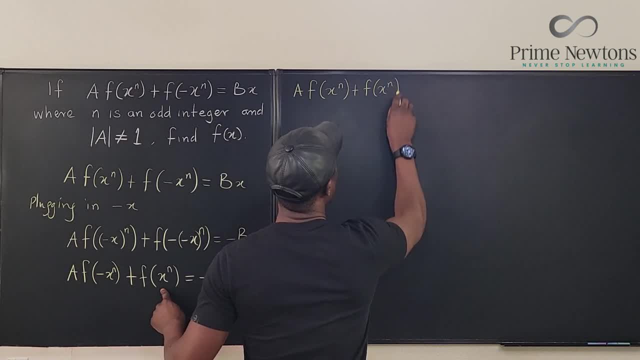 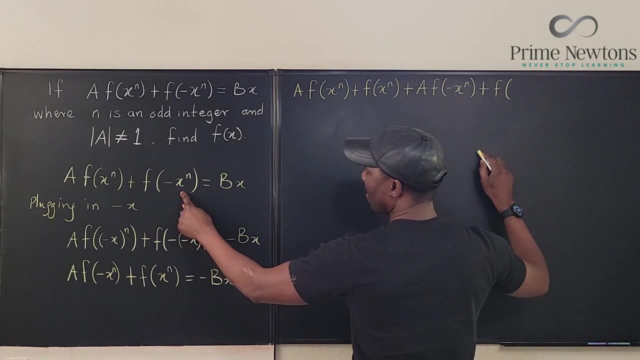 plus f of x to the n. Then I'm going to add this plus a times f of negative x to the n, or this one plus f of negative x to the n. Nice, We'll be equal to this plus this, which is equal to zero. 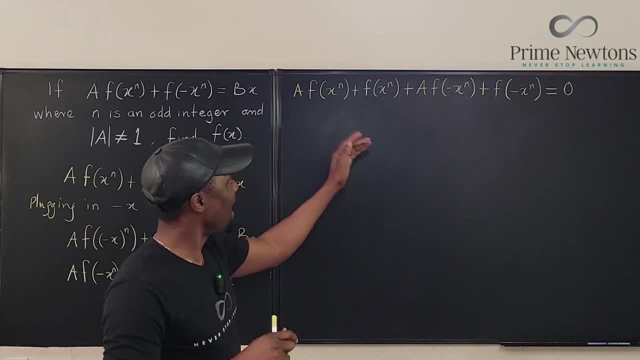 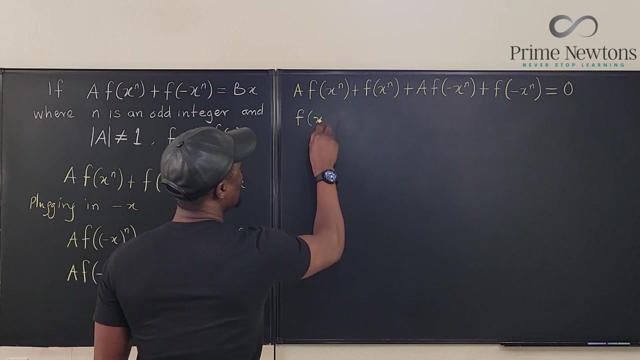 Now, just by writing out those lines, I can easily see that I can factor f of x to the n. So I have a. let's take out f of x to the n, f of x to the n. I'm going to be left with a. 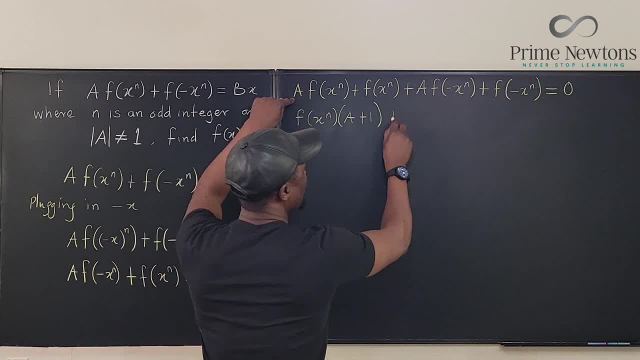 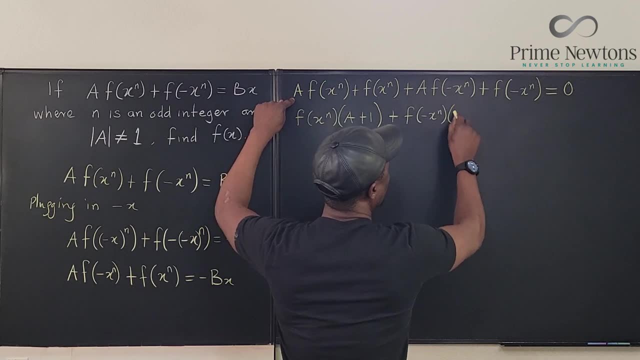 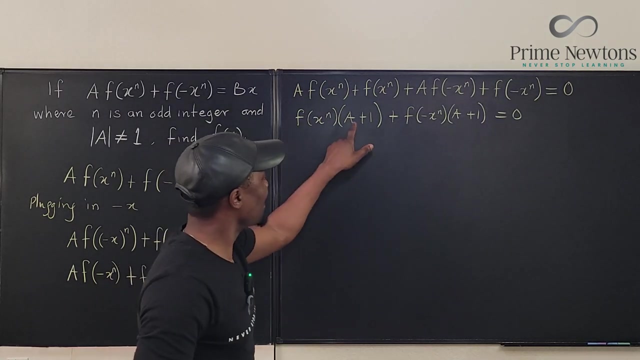 plus one from these two, And I'll do the same thing- plus f of negative x to the n. a plus one, Ooh, equals zero. So this looks like you factored a quadratic, So I can take out a plus one. So I have a plus one times f, nice x to the n, plus f of. 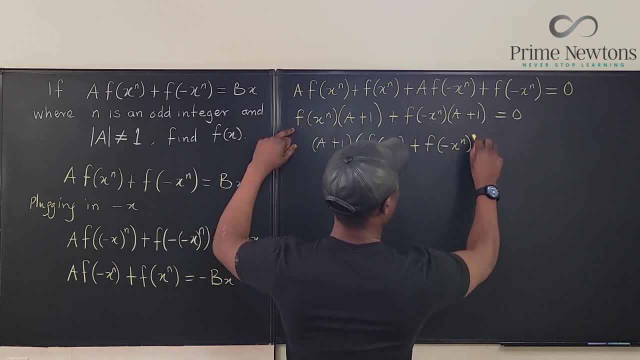 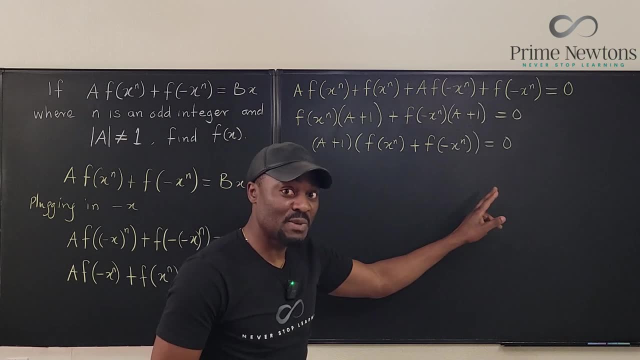 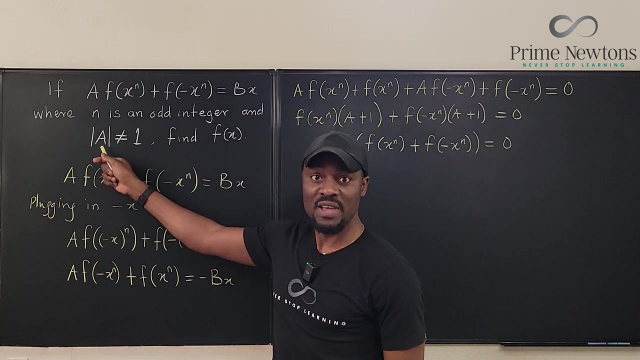 negative x to the n right there equals zero. Now, this is a product of two terms. One of them must be zero or both of them must be zeros. a plus one equals zero will mean a equals negative one. But we said the absolute value of a is not one. So we cannot, this cannot be zero. 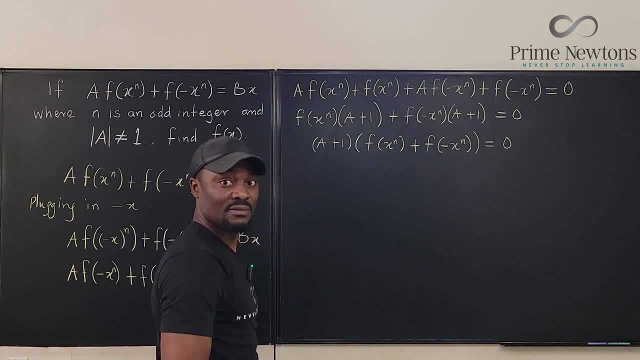 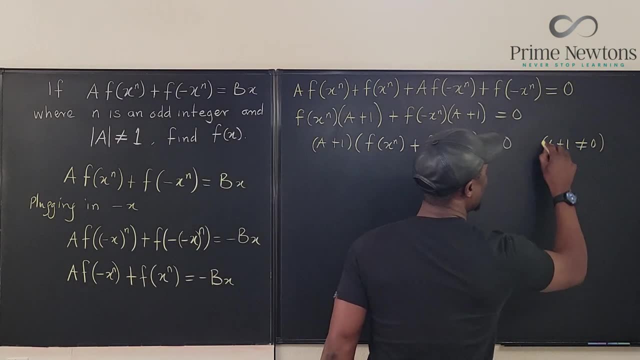 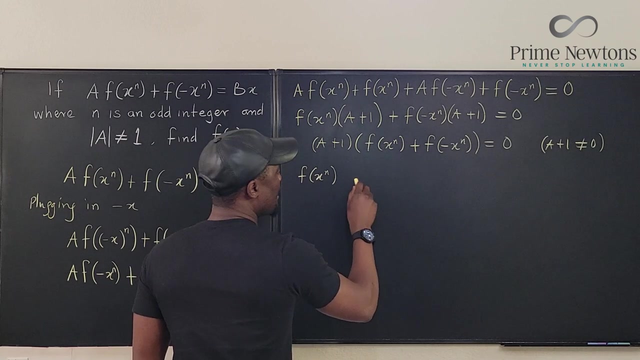 because of that, This has got to be our zero. Okay, So we know that a plus one is not equal to zero. So we're going to go here and say that f of x to the n plus f of negative x to the n. 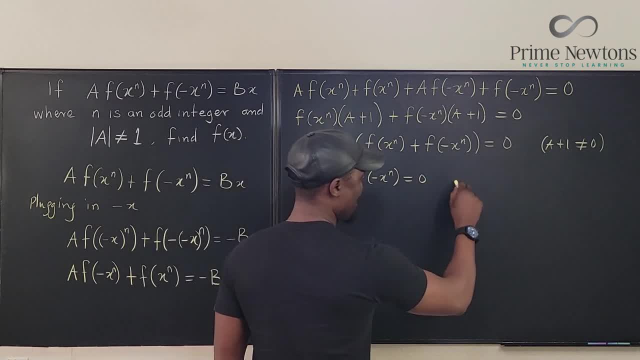 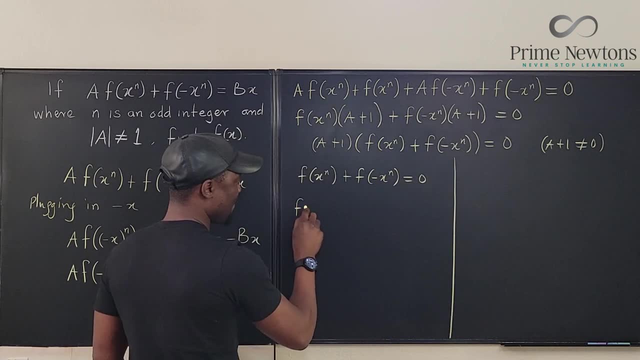 is equal to zero, Which means maybe I should go this way. Now let's, let's divide the board this way, Which means that f of x to the n equals negative f, negative x to the n, like that. So we move this over. Actually, I can move this minus sign because I can go replace this guy. 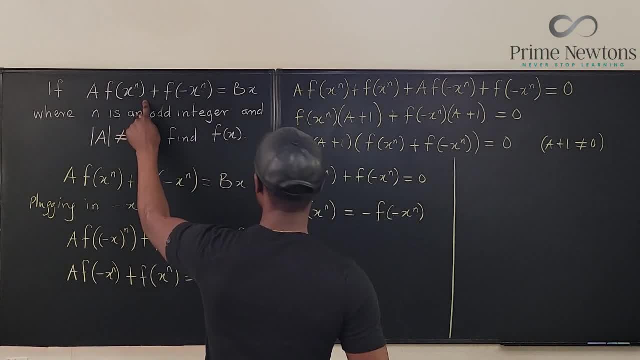 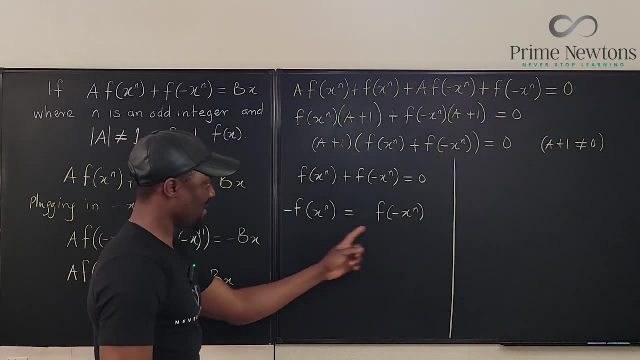 in the original equation. So I'm going to say that negative of this is this one. So if I go back to the original equation, ta-da-daaaahhhh. So here I have a times f of x to the n plus. 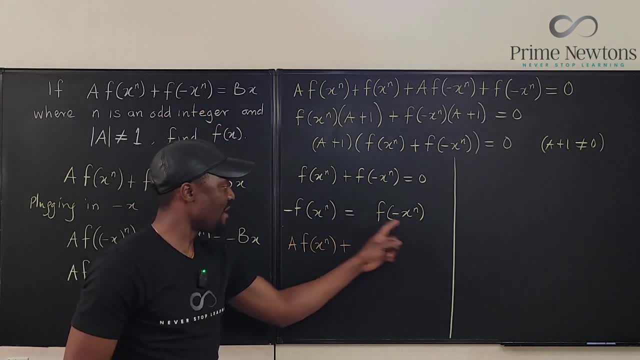 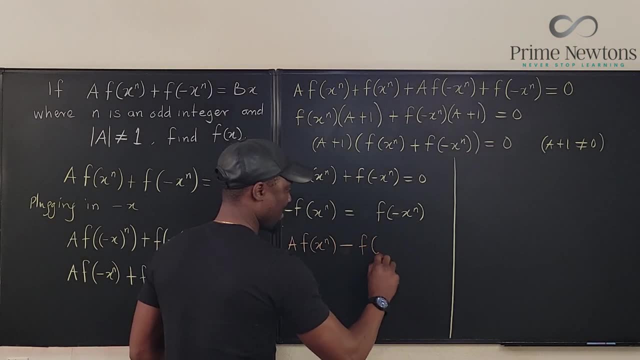 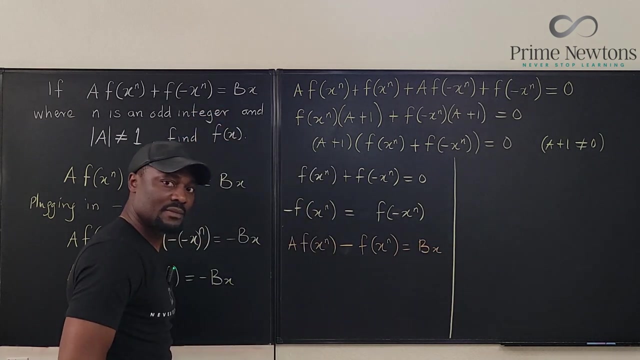 But instead of me adding this f of negative x to the n, I'm going to be adding this guy which is minus minus f of x to the n, equals bx. let me box this so you know that it's a different thing we're dealing with here. 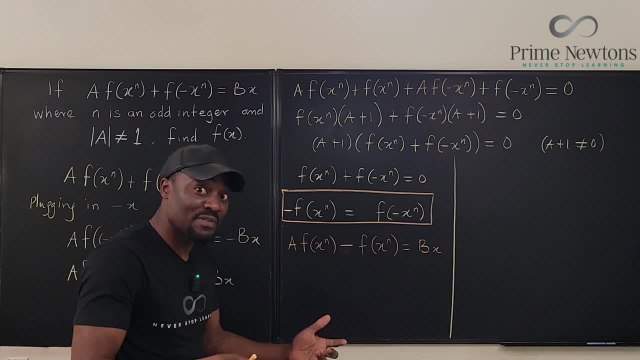 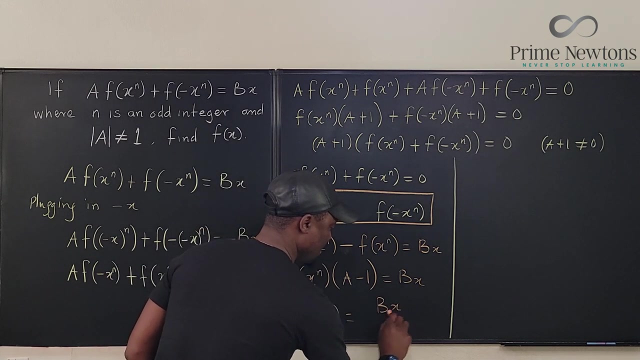 so what do i get here? remember, i'm looking for f of x, almost there. i can factor this out so that i have: f of x to the n times a minus 1 equals b x, so that f of x to the n equals b times x divided by a minus 1.